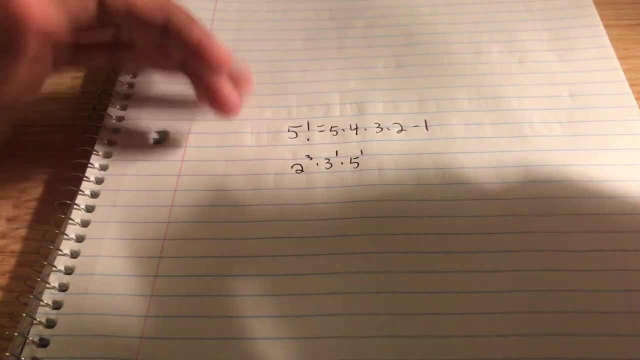 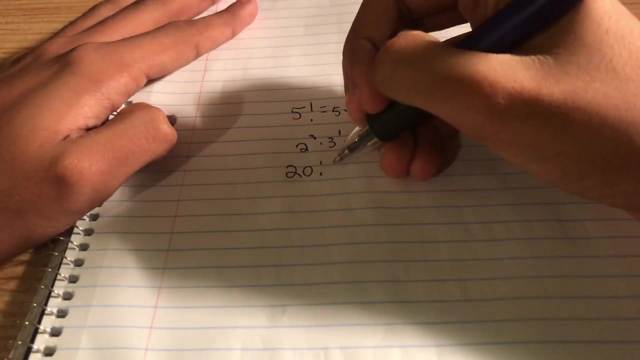 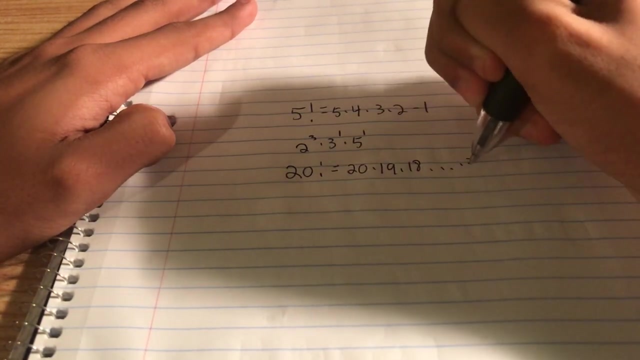 prime number within the factorial. So let's go to a little bit of a bigger example: 20 factorial. Okay. So obviously that's 20 times 19 times 18 times, 3 times 2 times 1, and stuff in between. 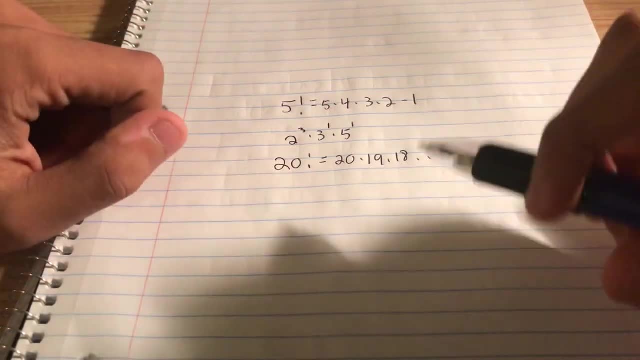 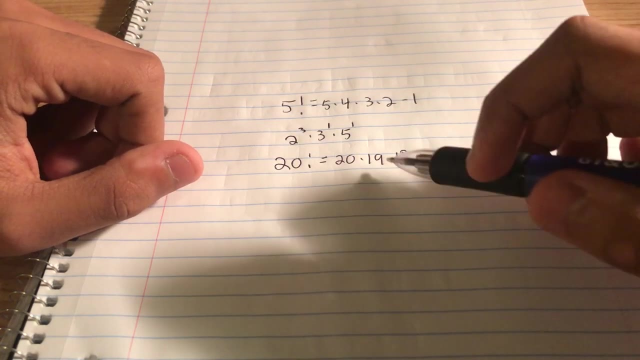 So let's just do what we did for 5: factorial: Start with the powers of 2.. Well, we can start with 2.. There's a 2 here, but then there will be a times 4.. then I times 6, 8, 10, 12, 16, 18, 20. each of those will have at least one power of 2. 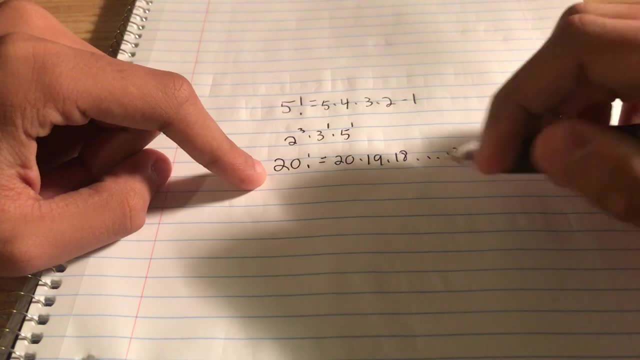 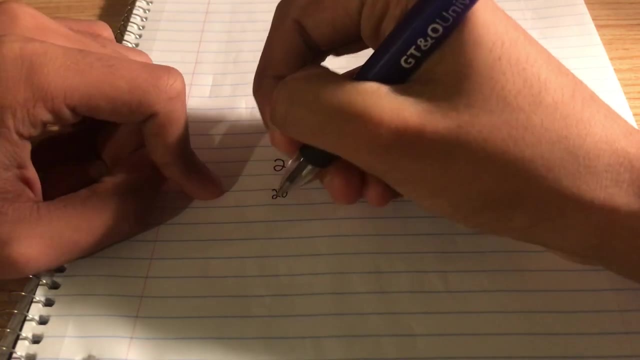 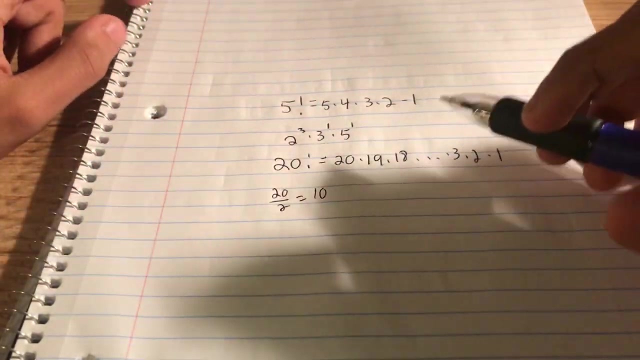 so we count up the number of twos, the number of twos in 20, so that's just 20 divided by 2, right? 20 divided by 2, so that's 10. so that's 2 to the power of 10. well, not exactly, keep in mind. 4 is 2 squared, so there's another power of 2 in. 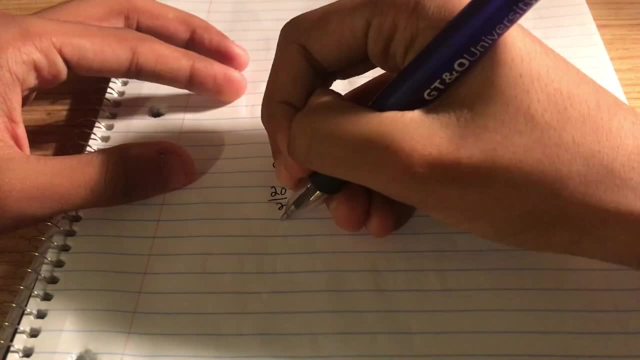 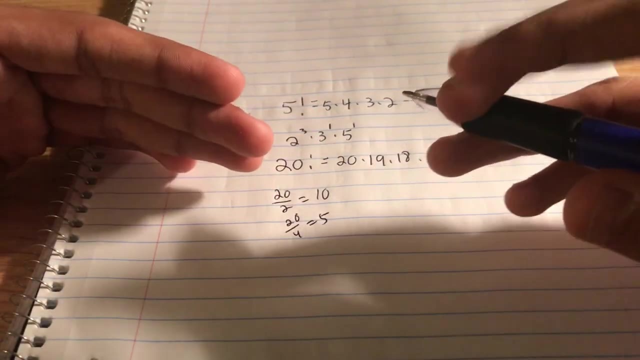 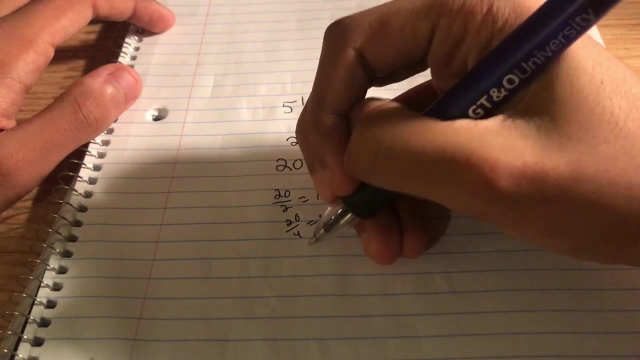 each multiple 4. so let's multiply 20 by 4 and we get. there are 5 more powers of 2. but hold on, there's also an 8. 8 is 2 cubed. so now we have to look at all the multiples of 8 up to 20. so if we do 20 divided by 8, we don't get an integer. 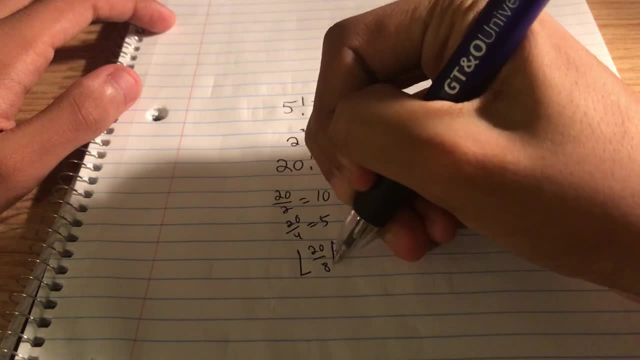 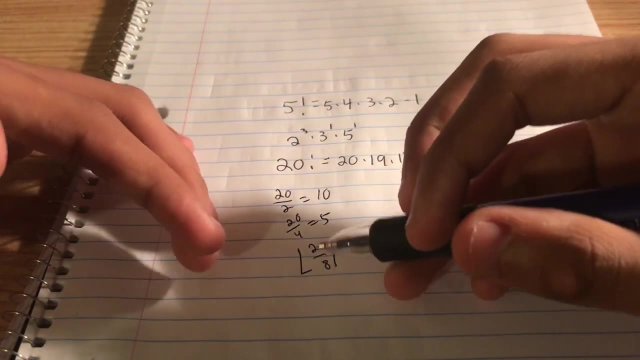 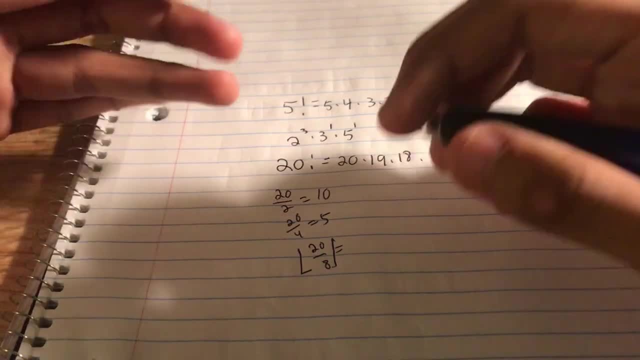 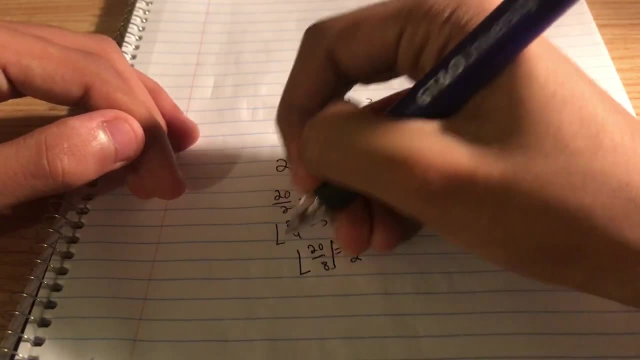 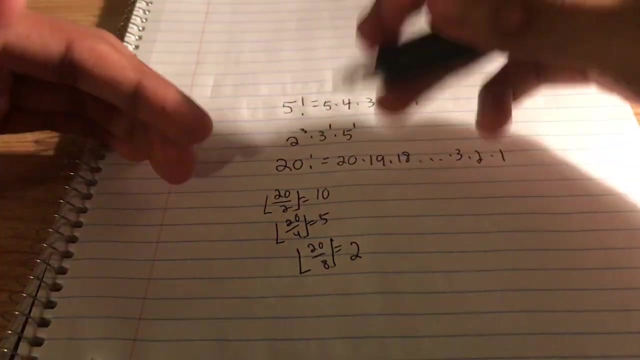 point something, right, 2 point something. but we don't want that point something, we just want a whole number. so round up down to 2. you always round down track. we can put floor functions on all of these, because of the floor function of an integer is just that integer: the floor function of that integer point. 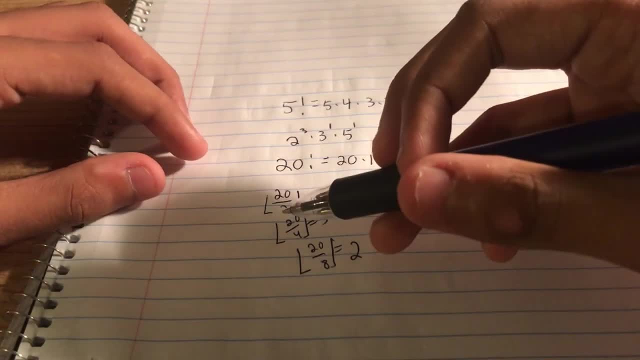 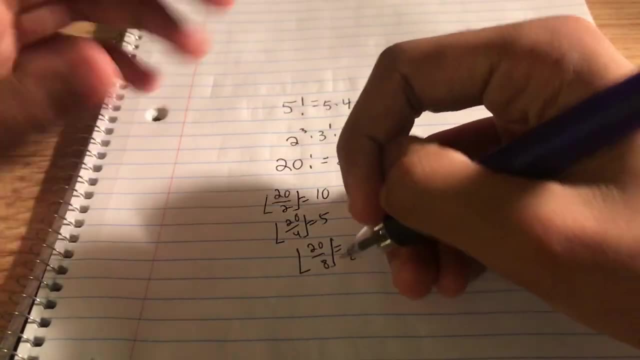 something is just that integer. so now we have the powers of 2, 4, 8 and all this. yeah, let's get rid of the 4, right, okay? so this is an integer. so this is the number of powers of 2 in 20 is 2 squared, so that gives us a total of 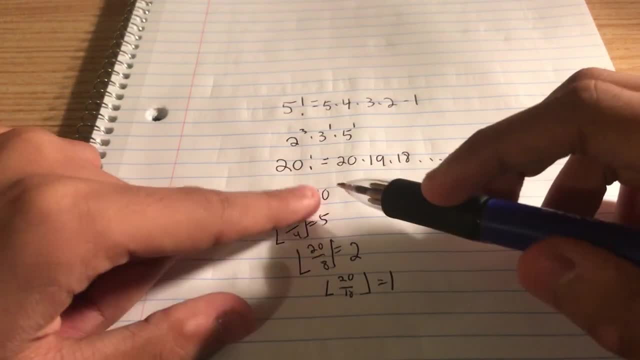 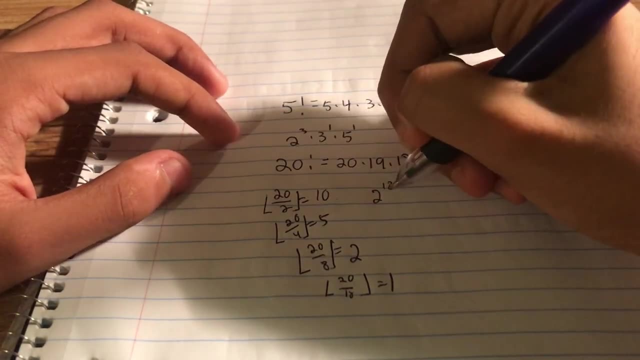 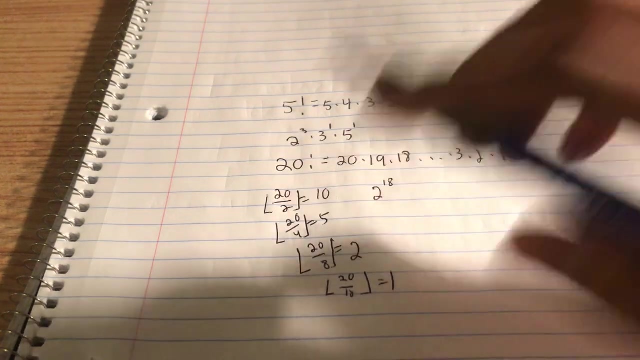 1, as we the number of powers 2 squared, and what we get is 2 squared, so that gives us the total of 16.. oh, don't forget 16. 16 is 2 to the power of 4, so there's an extra power of 2 there. so 20 divided by 16, the for that is equal to 1. 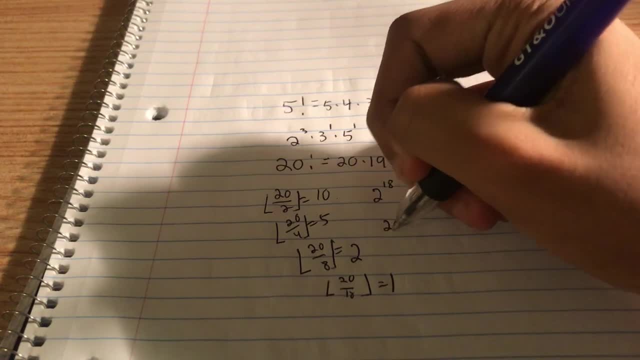 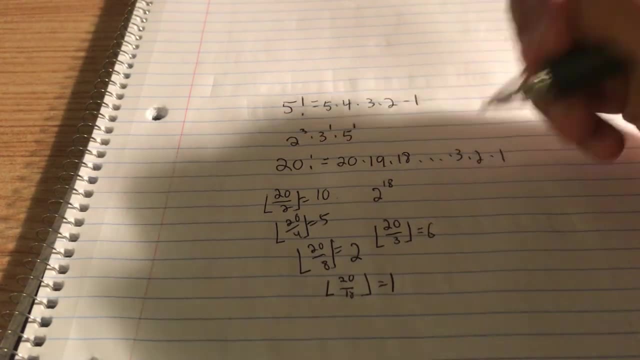 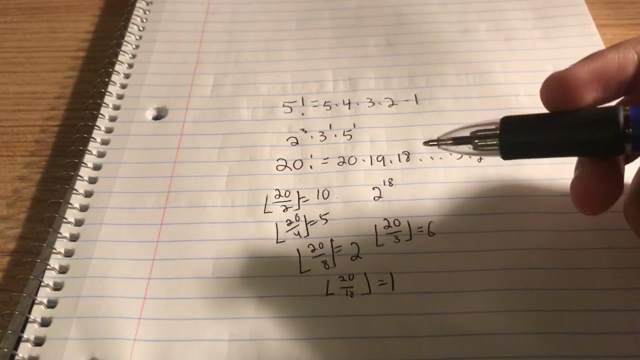 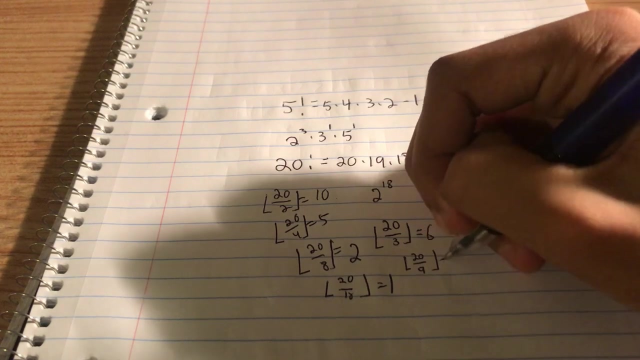 one power of 3 num. so let's do 20 divided by 3, forward forward, so that equals 6. so you got at least 6. then you got, let's see, 9. 9 is 3 squared, correct. so let's look at the multiples of 9 up to 20. so the floor function of 20 divided. 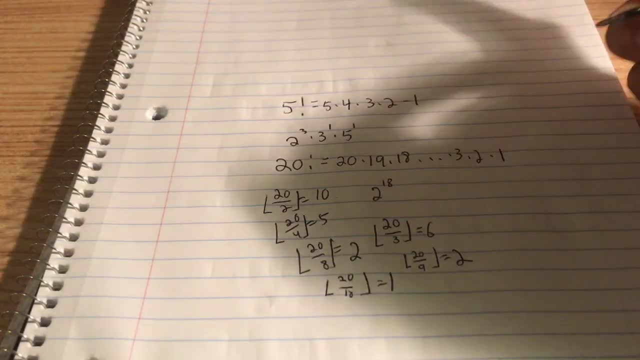 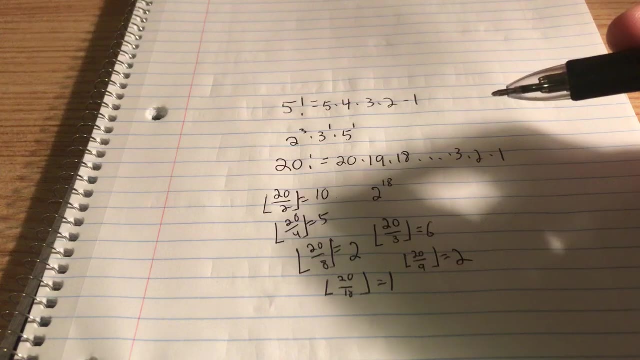 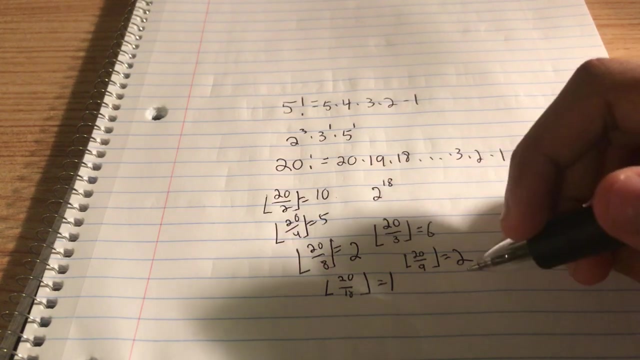 by 9 is 2. now, is there anything else? well, 3 squared is 9. what's 3 cubed? well, that's 27, and 27 is bigger than 20. so we don't need to check any more powers of 3. we already have this many. 6 plus 2, that's 8. so it's 2 to 18 times 3 to the. 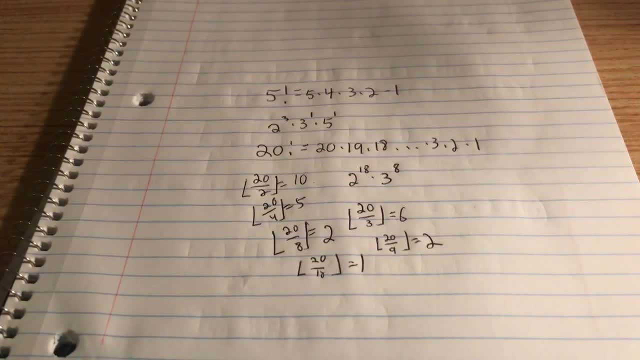 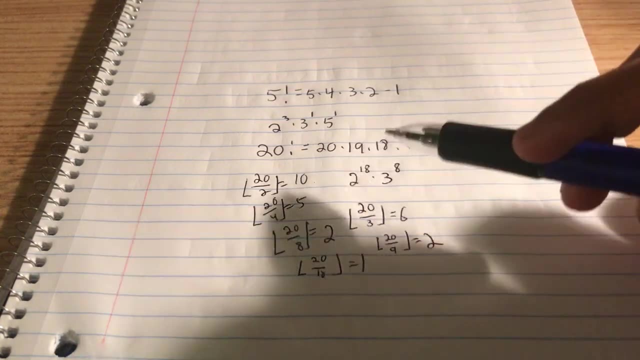 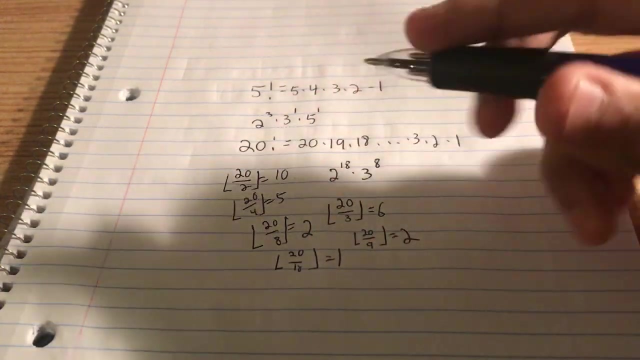 8th. so let's check now the next prime, which is 5, not 4. remember we don't need to check non prime numbers. this is prime factorization, so we're doing this for each prime number. remember that. so let's check 5. 5, 10, 15, 20. those multiples of 5 are under or equal to 20. 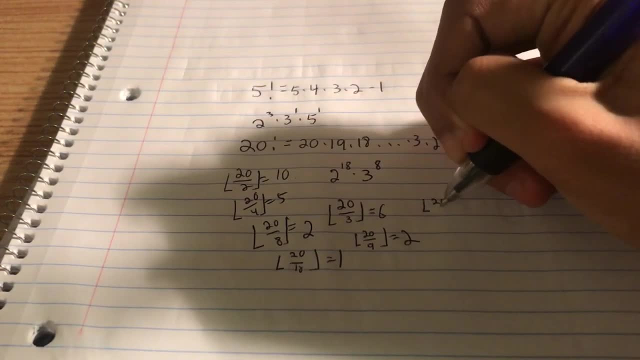 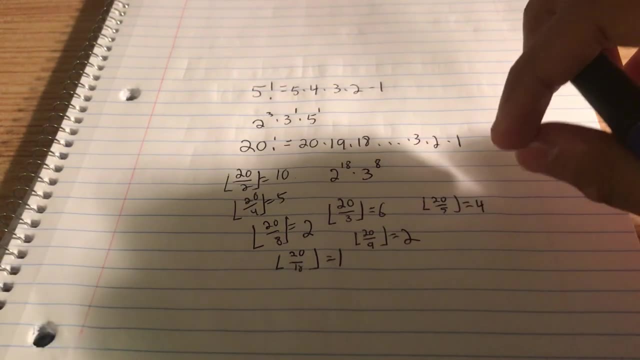 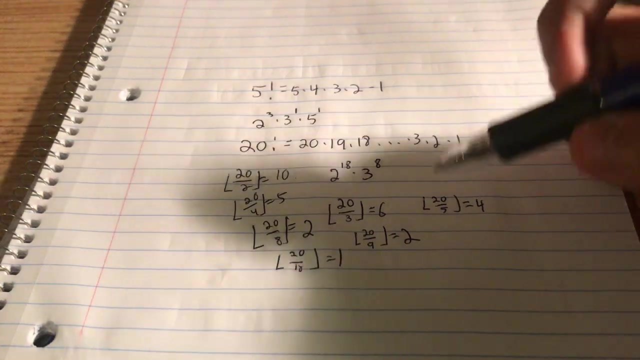 and have at least one power of 5. so let me just write it over here: 20 divided by 5 is equal to 4, so there's at least 4 powers of 5. now what about 5 squared? well, 5 squared is 25, and 25 is bigger than 20. so we don't have to go. 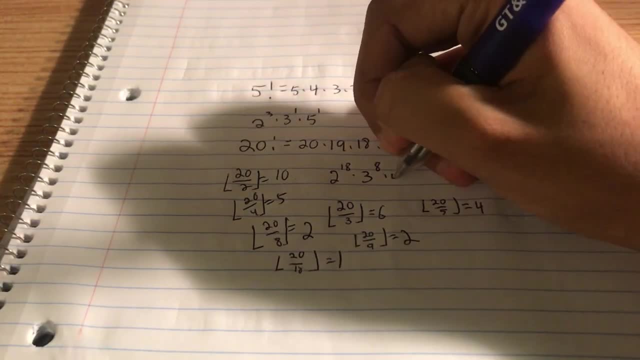 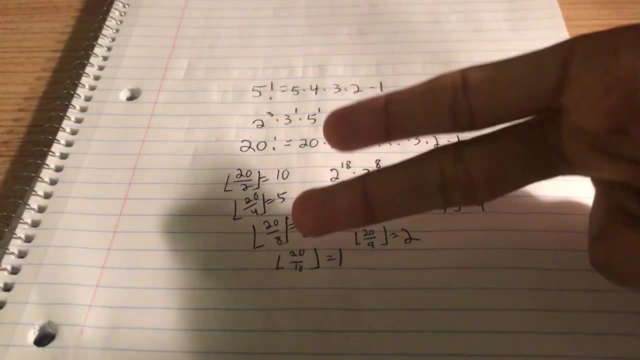 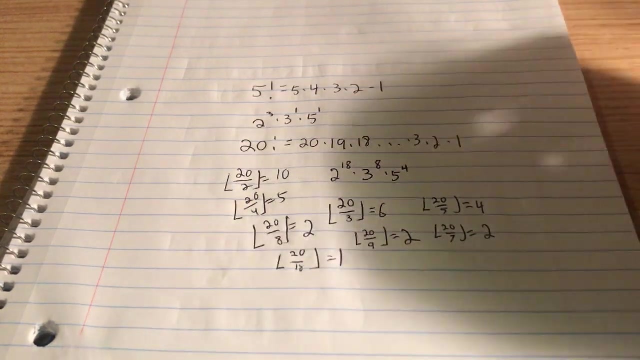 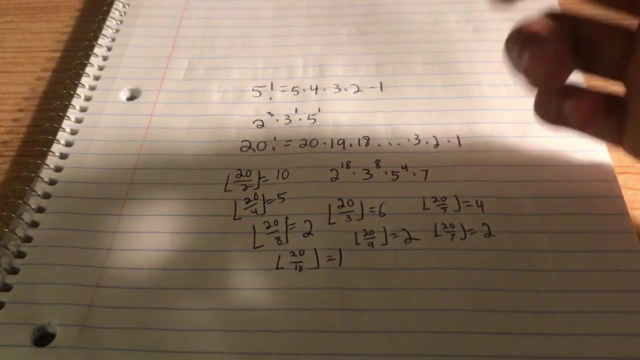 anywhere else. we can just write it over here, so we don't have to go anywhere else. so we don't have to go anywhere else. so we don't have to go anywhere else. but 7 squared is 49, which is already way bigger than 20, right? so it's not gonna. 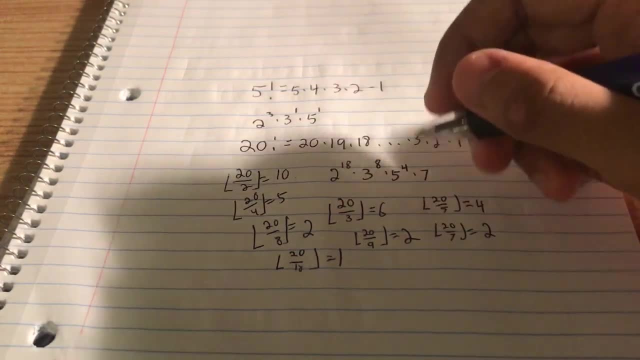 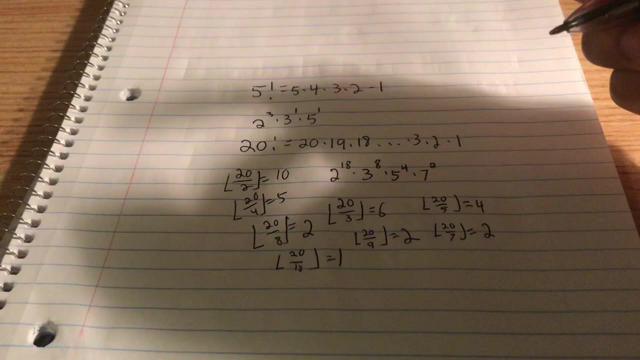 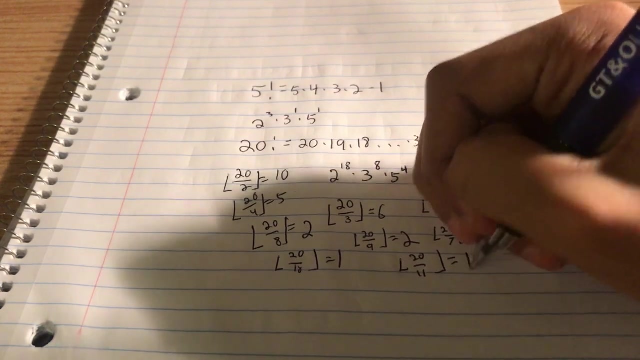 be anywhere near that proximity in which we're gonna have another power of 7. so So there's a 7 squared. Let's see 8 is not prime, 9 isn't prime, 10 isn't prime 11.. Well, the floor of 20 divided by 11 is 1 point something, aka just 1.. 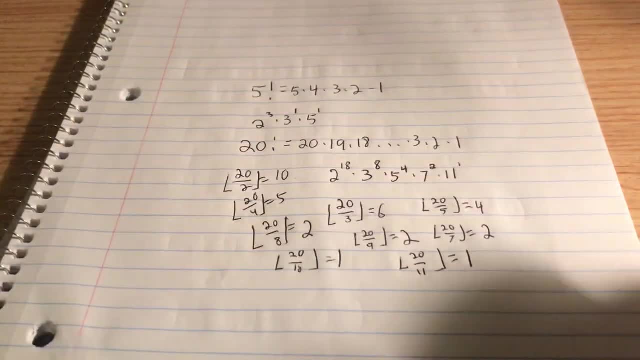 So there's just 1 power of 11. And again, we don't have to look for 11 squared, because 11 squared is 121, which is 101 bigger than 20. So we don't have to worry about that. 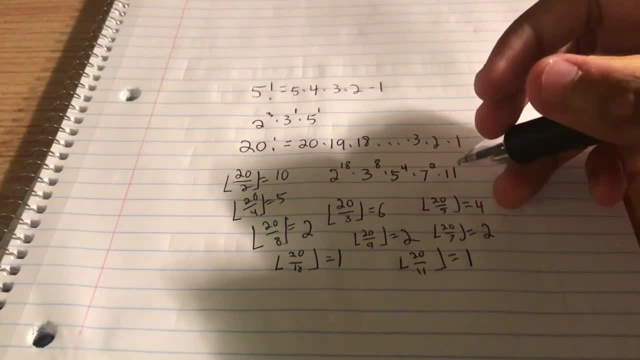 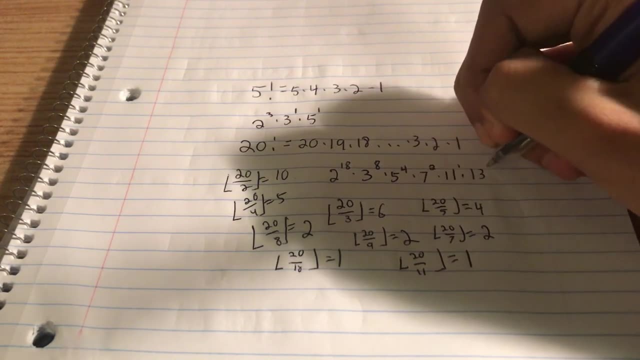 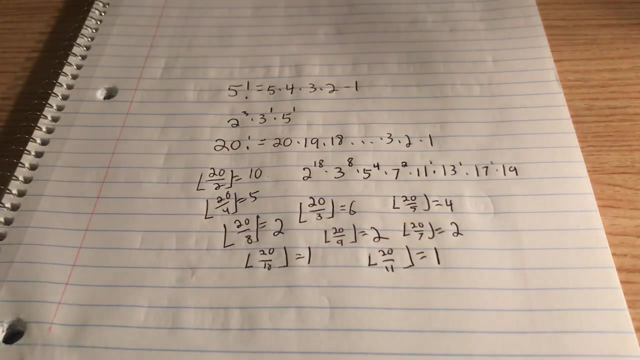 So now, from now onwards, every prime is only going to have 1,, because the square of that prime is going to be so much bigger than 20.. So let's see what's the next prime: 13,, let's see 17,, 19, and no more, because the next prime number is 23.. 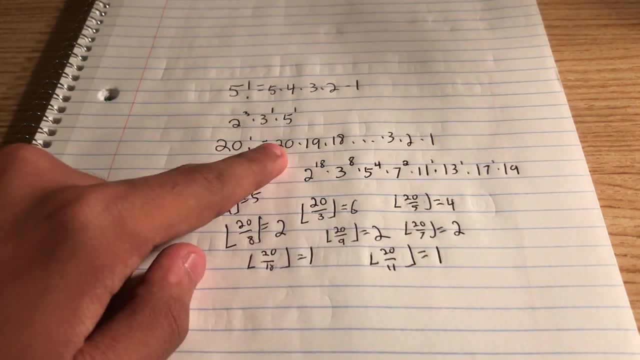 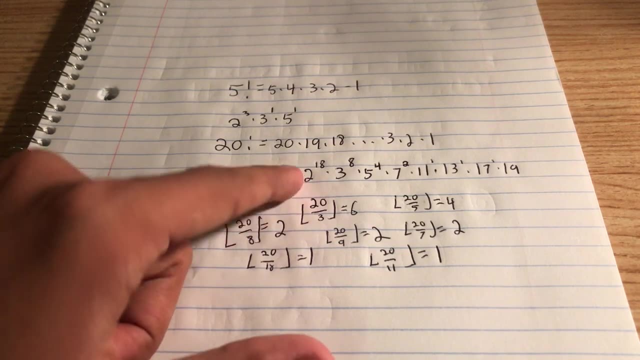 But 23 is bigger than 20.. And obviously 23 is not in 20 factorial. You can't make a 23 in 20 factorial. So this is it. This is our whole prime factorization 2t at.